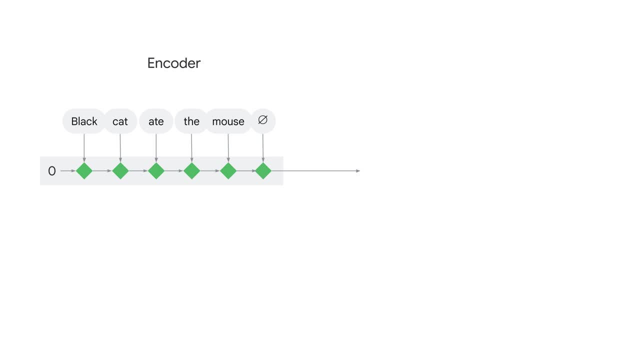 target language. Here's an example. Take this sentence: black cat ate the mouse. In this example, the first English word is black. However, in the translation the first French word is che, which means cat in English. So how can you train a model to focus more on the word cat instead of the word black? 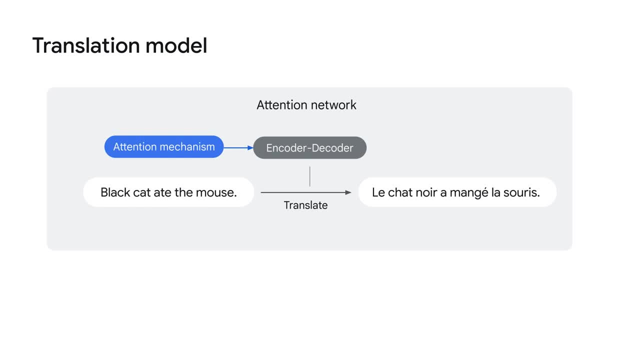 Well, the answer is simple: You need to be able to Sale at the first time-step, and モ- My mind is fooling me. if there is one way of saying the disappear of the verb my. You can learn to do this to find solutions for using LLM models. You can give a lecture on what is called the attention mechanism. In fact, the importance of this voice command to cram in your아요 your own speech is to make it accessible to your own typing skills, and then, best です are speaking to the provider or your你们 like, producing the對 track. 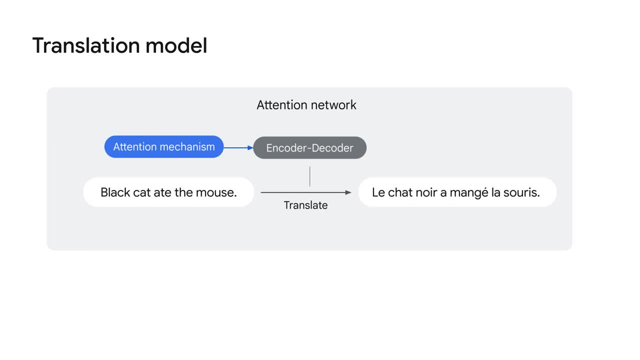 Atention mechanism is a technique that allows the neural network to focus on specific parts of an input sequence. This is done by assigning weights to different parts of your input sequence, with the most important parts of receiving the highest weight you wouldбу like to get. After you get 2 levels, 1 less or even 2 parts of your normal speech. 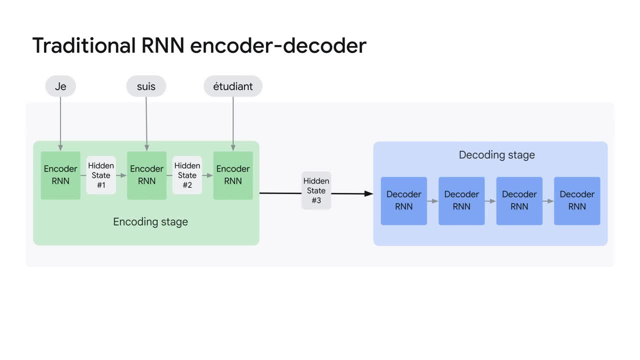 This is what a traditional RNN-based encoder-decoder looks like. The model takes one word at a time as input updates the hidden state and passes it on to the next time step. In the end, only the final hidden state is passed on to the decoder. 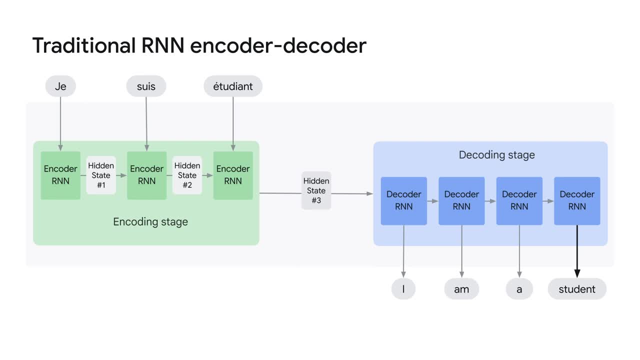 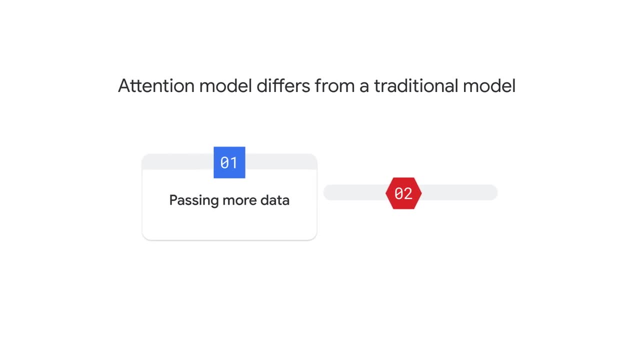 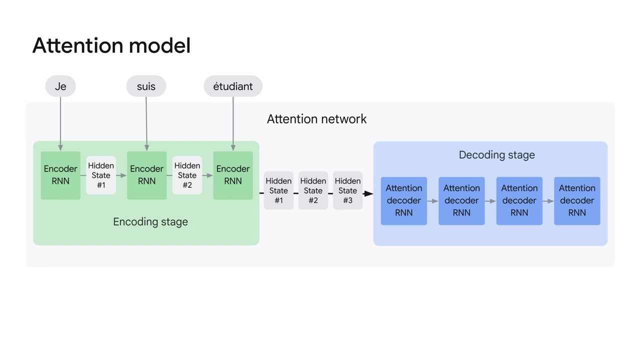 The decoder works with the final hidden state for processing and translates it to the target language. An attention model differs from the traditional sequence-to-sequence model in two ways. First, the encoder passes a lot more data to the decoder. So instead of just passing the final hidden state- number 3, to the decoder, the encoder passes all the hidden states from each time step. 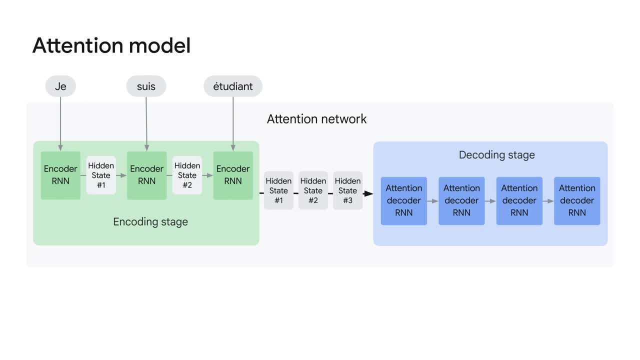 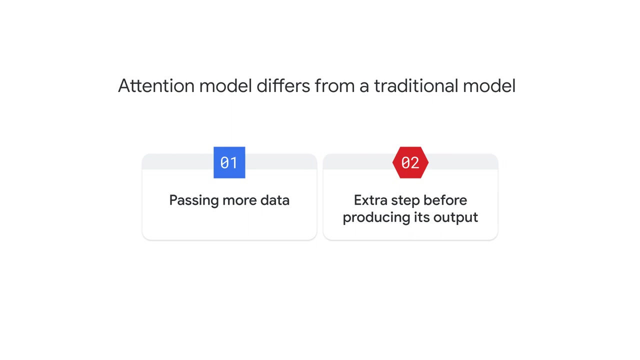 This gives the decoder more context beyond just the final hidden state. The decoder uses all the hidden states to pass the final hidden state. The decoder uses all the hidden state information to translate the sentence. The second change that the attention mechanism brings is adding an extra step to the attention decoder before producing its output. 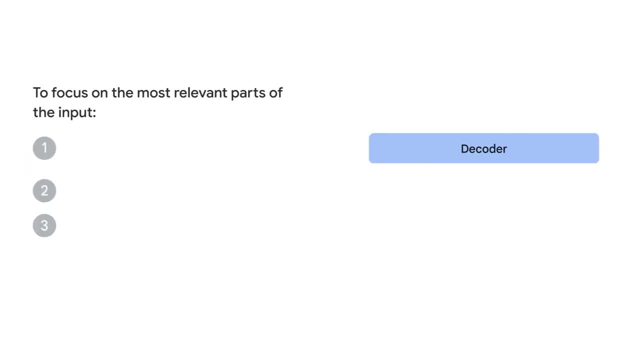 Let's take a look at what these steps are, To focus only on the most relevant parts of the input. the decoder does the following. First, it looks at the set of encoder states that it has received. Each encoder state has a set of encoder states. 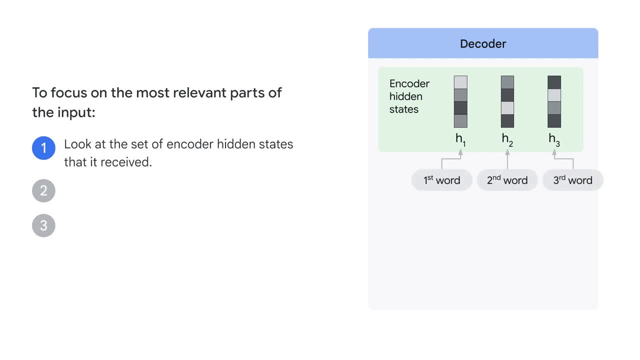 Each encoder hidden state is associated with a certain word in the input sentence. Second, it gives each hidden state a score. Third, it multiplies each hidden state by its softmax score, as shown here, Thus amplifying hidden states with the highest scores and downsizing hidden states with low scores. 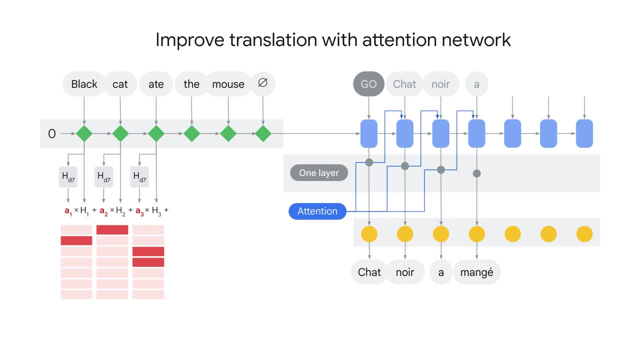 If we connect all of these pieces together, we're going to see how the attention network works. Before moving on, let's define some of the notations on this slide. Alpha here represents the attention weight at each time step. H represents the hidden state of the encoder RNN at each time step. 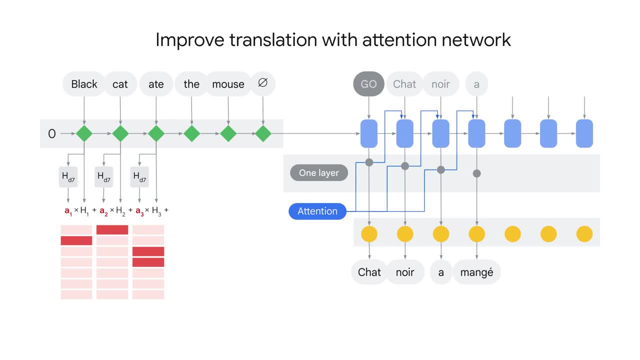 H, subscript D represents the hidden state of the decoder RNN at each time step. With the attention mechanism, the inversion of the black cat translation is clearly visible in the attention diagram. With the attention mechanism, the inversion of the black cat translation is clearly visible in the attention diagram. 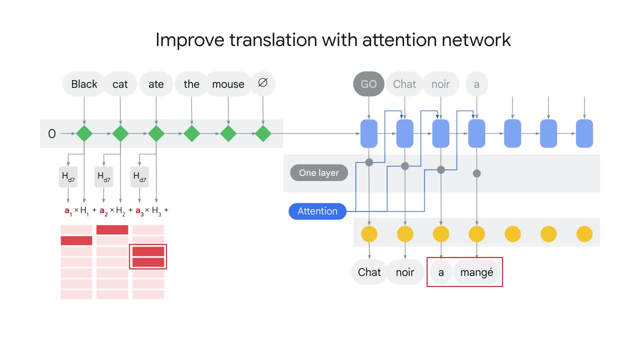 And eight translates as two words: imager and French. We can see the attention network staying focused on the word eight for two time steps. During the attention step we use the encoder hidden states and the H4 vector to calculate a context vector A4 for this time step. 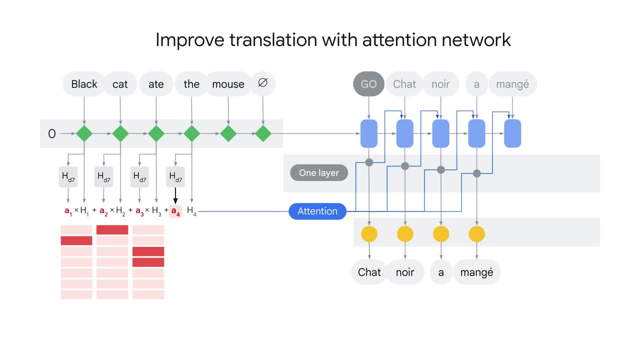 During the attention step, we use the encoder hidden states and the H4 vector to calculate a context vector A4 for this time step. This is the weighted sum. We then concatenate H4 and A4 into one. We then concatenate H4 and A4 into one. 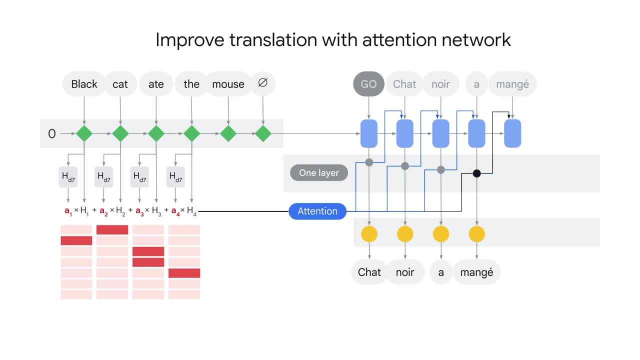 We then concatenate H4 and A4 into one vector. This concatenated vector is passed through a feedforward neural network, one trained jointly with the model, to predict the next word. The output of the feedforward neural network indicates the output word of this time step. 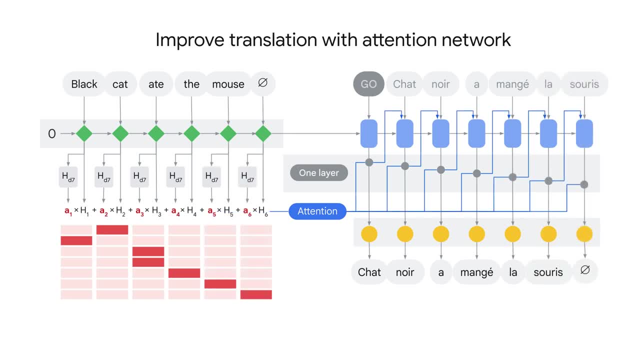 This process continues till the end of sentence. token is generated by the decoder. This is how you can use an attention mechanism to improve the performance of the decoder. This is how you can use an attention mechanism to improve the performance of the decoder. This is how you can use an attention mechanism to improve the performance of a traditional encoder-decoder architecture.